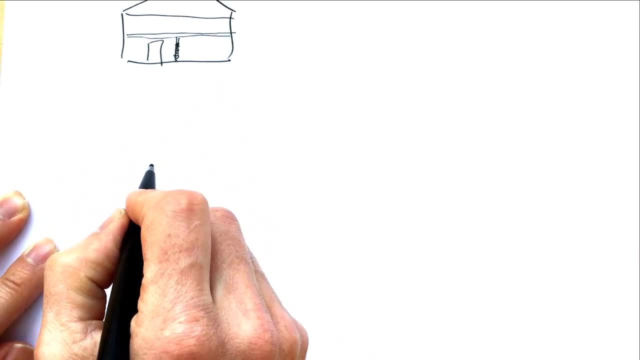 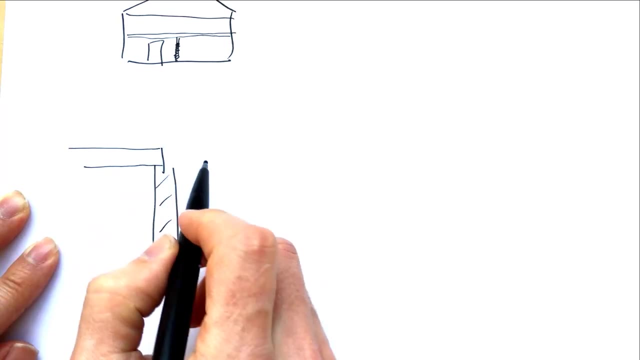 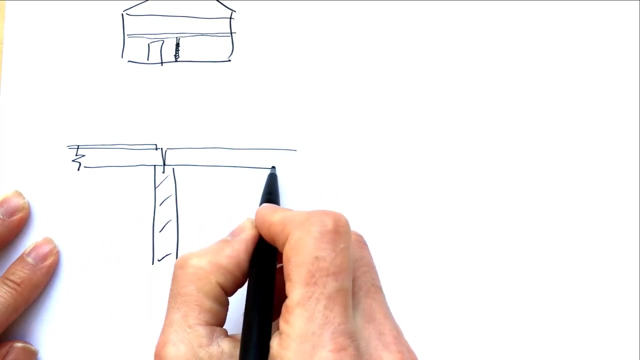 Now, if we zoom in here a little bit, there's an existing wall and it's got a floor sitting on it, And on the other side it's got the floor from another room sat on it And we're also going to imagine that the wall carries on up. 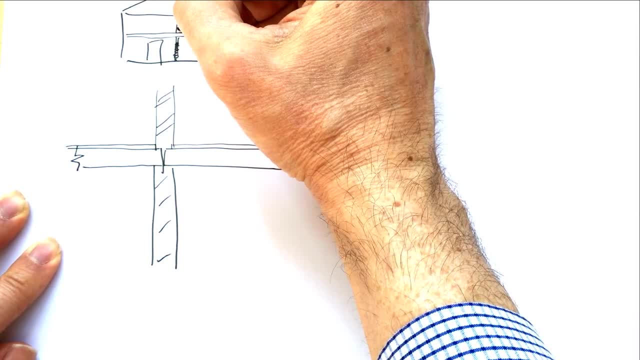 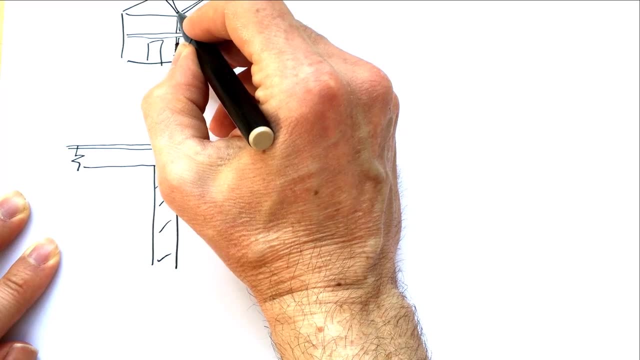 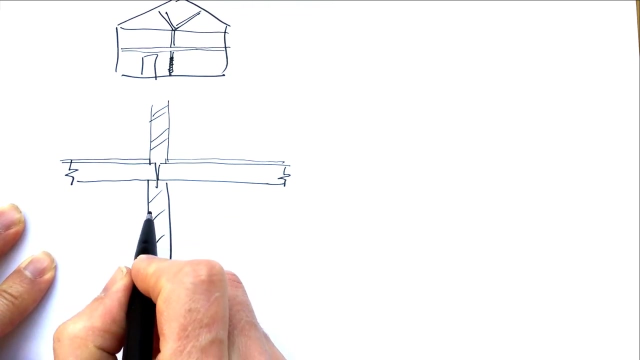 Through the first story And let's just imagine that there's a roof which is braced and also sitting on there. So if we knock this wall out, we're going to have to put a steel beam in there to support it, Because this has now disappeared. 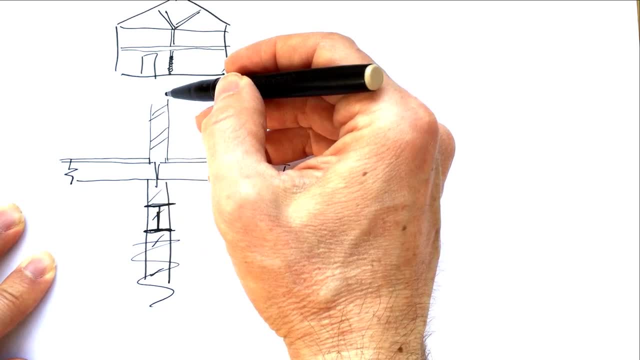 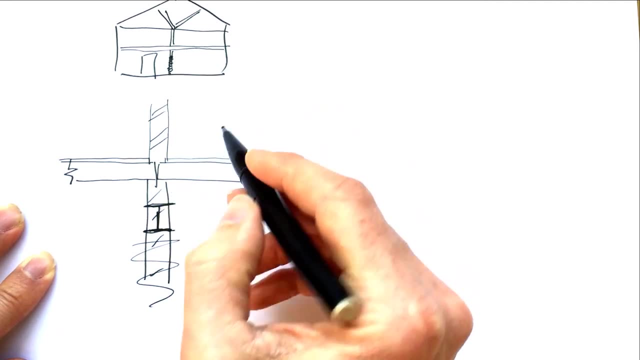 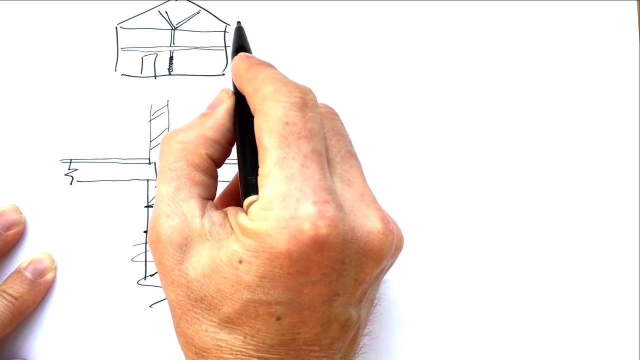 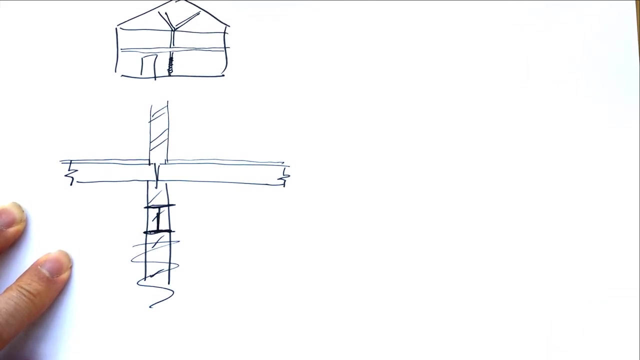 So the load on that beam is going to be a certain height of masonry, brickwork or blockwork And it's going to be a certain span of floor and a certain span of roof. So loadings are very simple. You're going to have to look in the 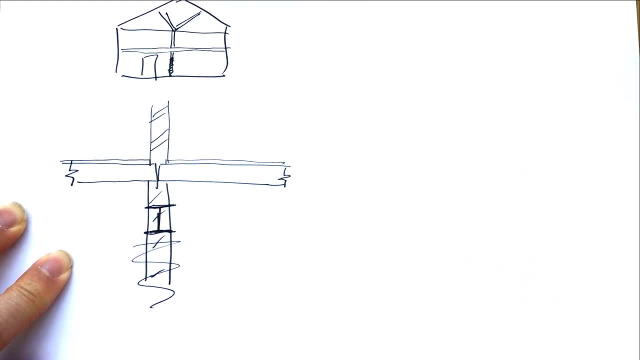 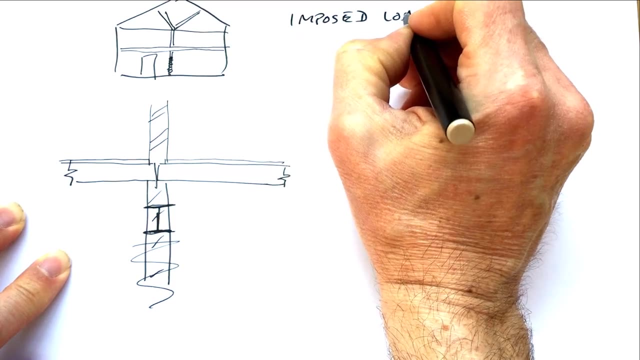 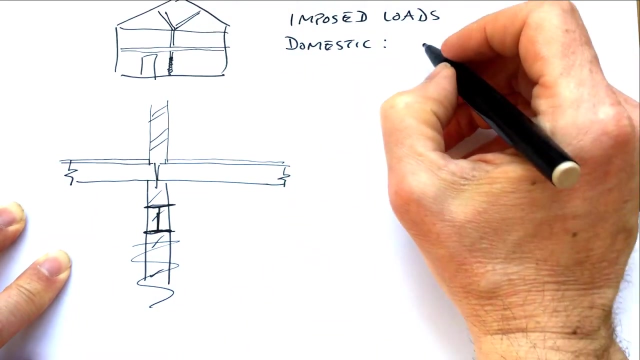 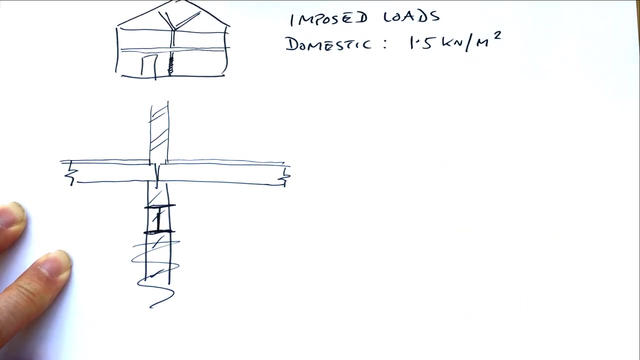 tables of loads for your particular country And you will find on there imposed loads for domestic situations And in the UK 1.5 kilonewtons per meter squared is the required imposed load for a domestic floor. There is also going to be the weight of the floor. 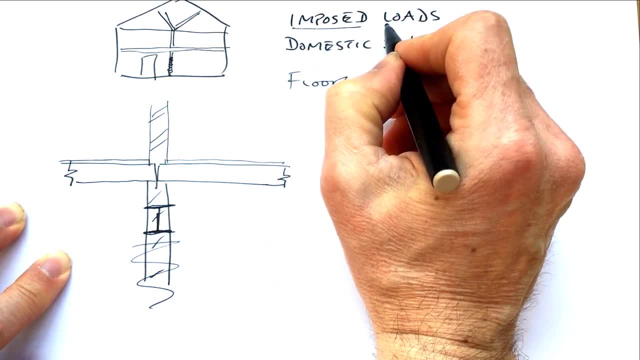 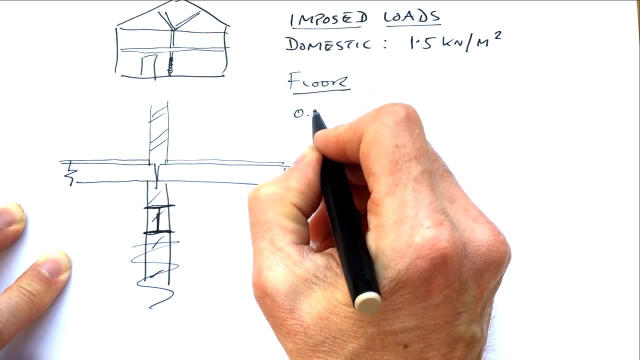 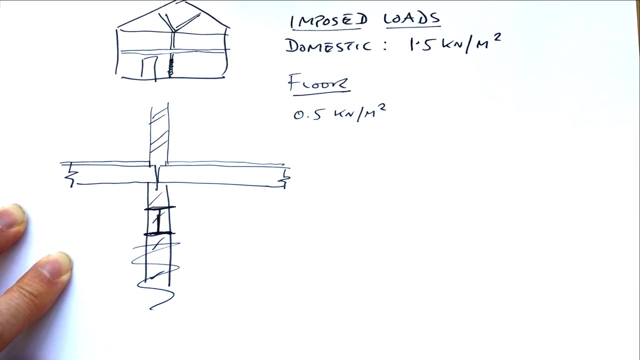 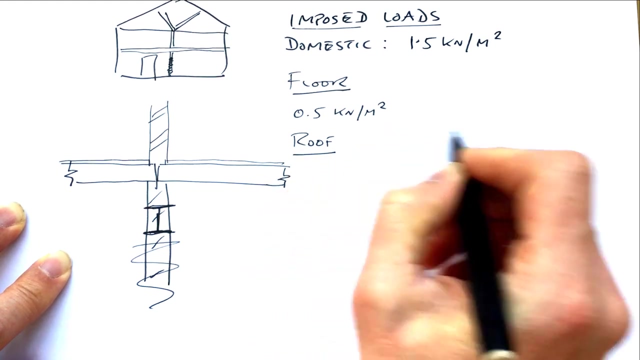 Which in this case, we're going to take as 0.5 kilonewtons per meter squared, And that's a usual, quite an average, load for a timber floor. The roof is likely to come in at about 1 kilonewton per meter squared. 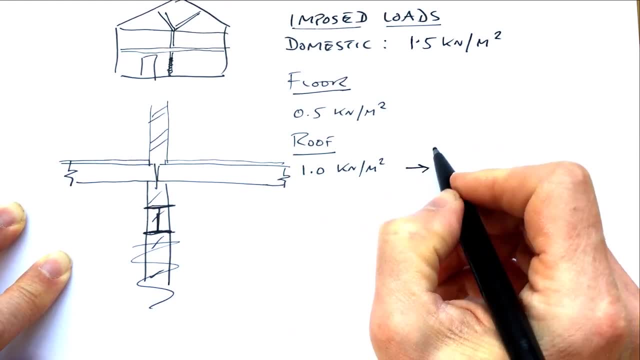 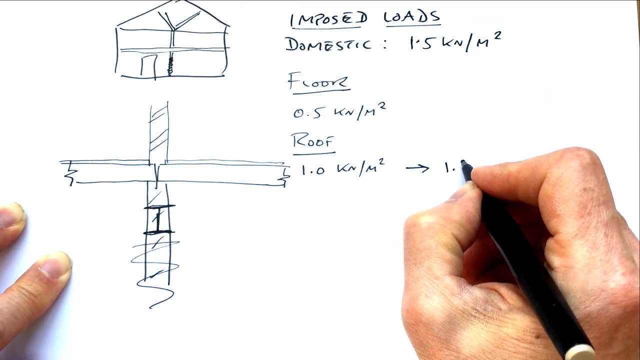 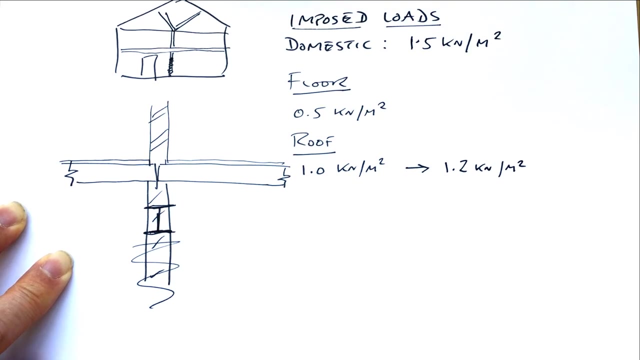 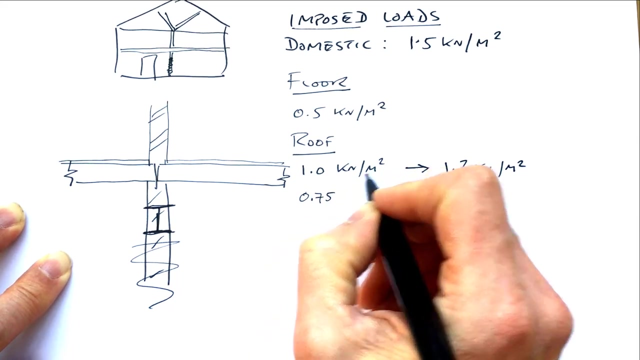 And by the time we've taken into account the fact that everything is on a pitch, we'll take it as 1.2 kilonewtons per meter squared, And the roof is also going to have an imposed load because of potential snow. 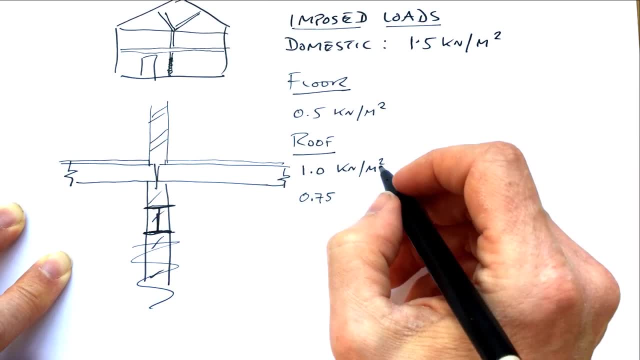 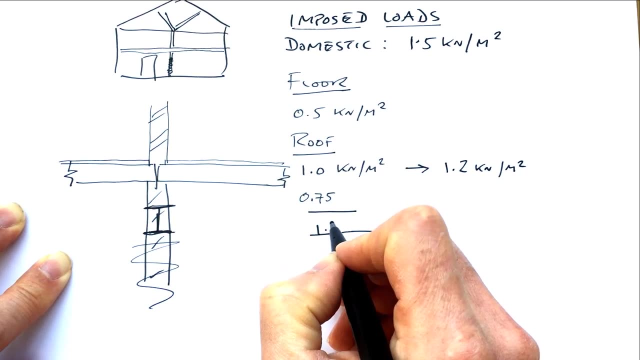 people accessing the roof and wind, which is 0.75.. So the total for the roof will be one point. let's say 1.2 plus 0.75, let's say 2 kilonewtons per meter squared. 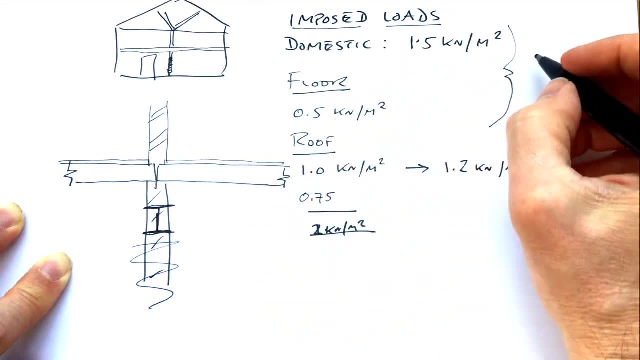 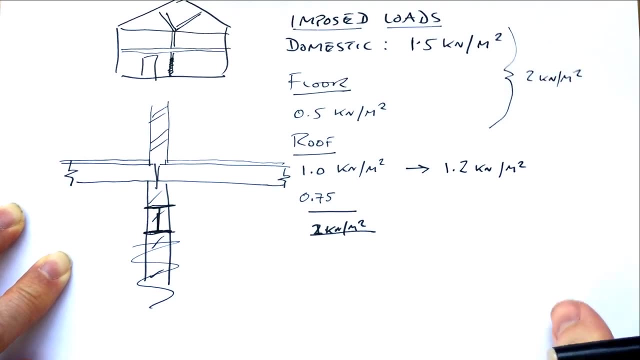 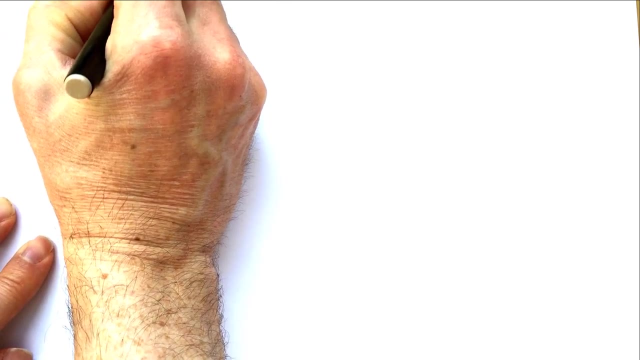 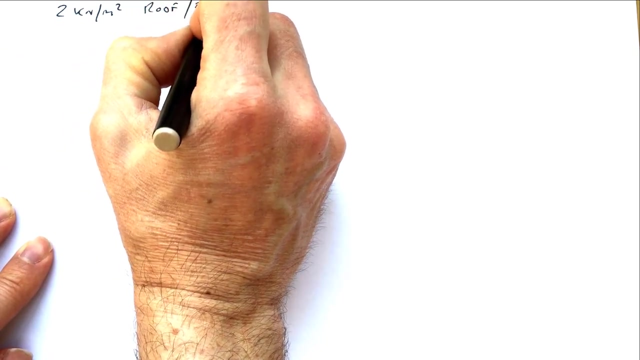 And for the floor also, 1.5 plus 0.5 is 2 kilonewtons per meter squared. So the loadings we've got is 2 kilonewtons per meter squared for a roof or a floor. 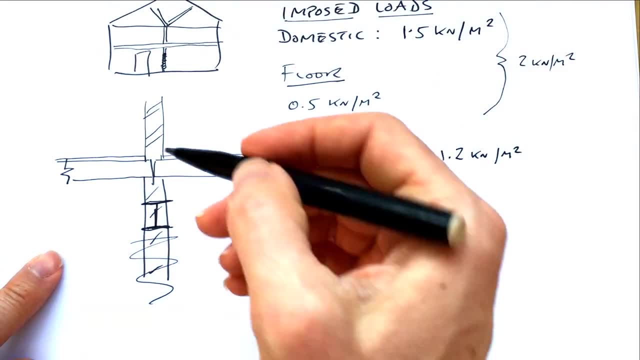 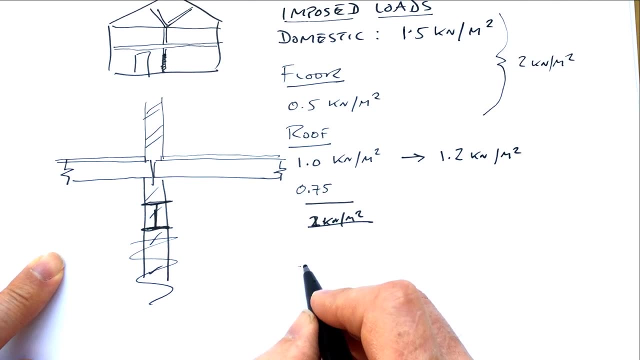 And for a wall, this wall sitting on here we're going to take. I'll work it out here for you. so it's roughly 20 kilograms- sorry, it's roughly 20 kilonewtons per meter cubed and it's roughly 0.1 meter thickness. 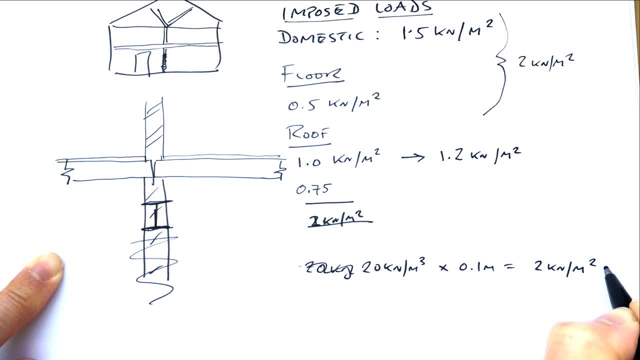 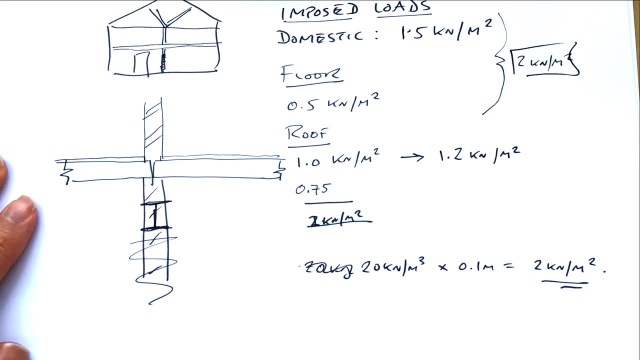 So again, 2 kilonewtons per meter squared. So the method I'm showing you is very, very easy to remember, because it's 2 kilonewtons per meter squared for a floor, 2 kilonewtons per meter squared for a roof. 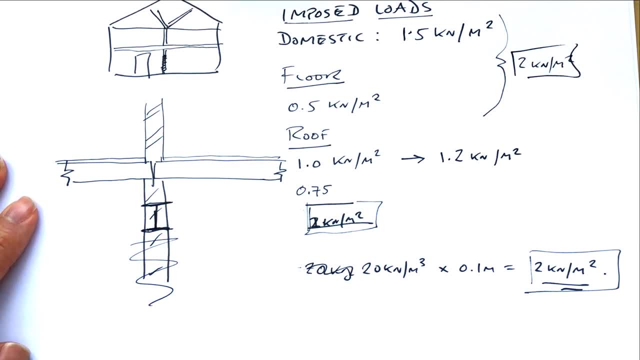 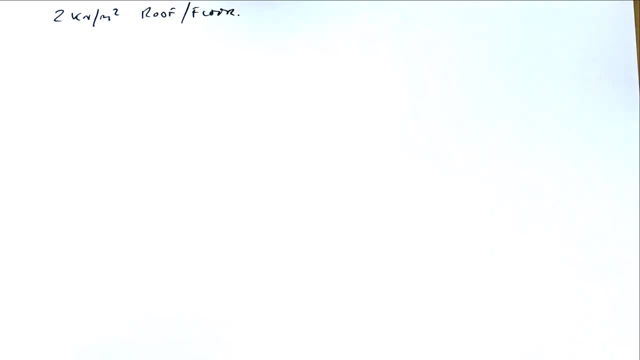 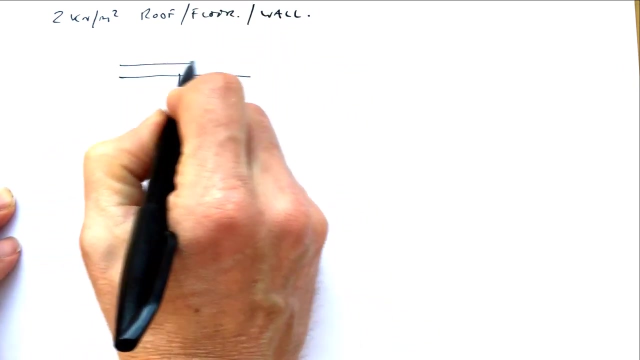 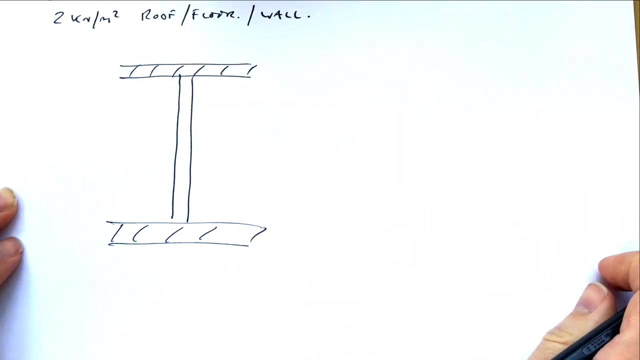 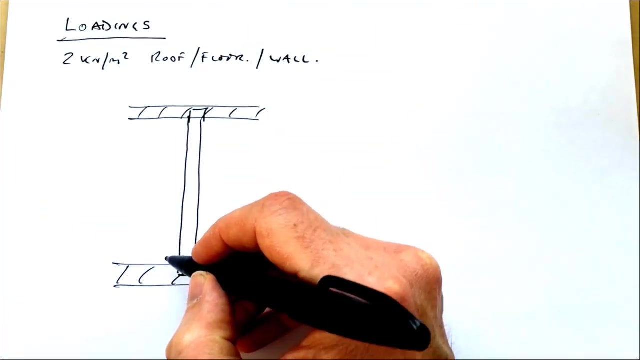 and 2 kilonewtons per meter squared for a wall. Now we're going to draw this on plan. Here's your beam, There's one supporting wall and there's another supporting wall. As an aside, you must check that there doesn't need to be. 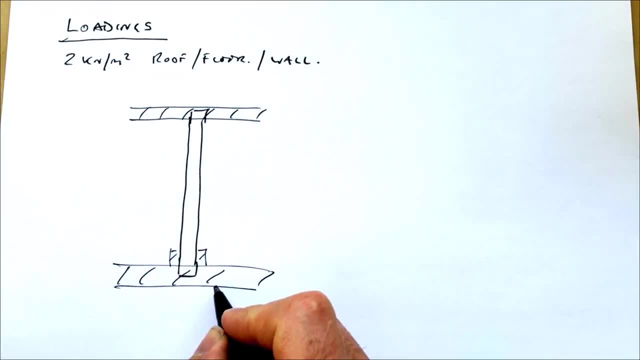 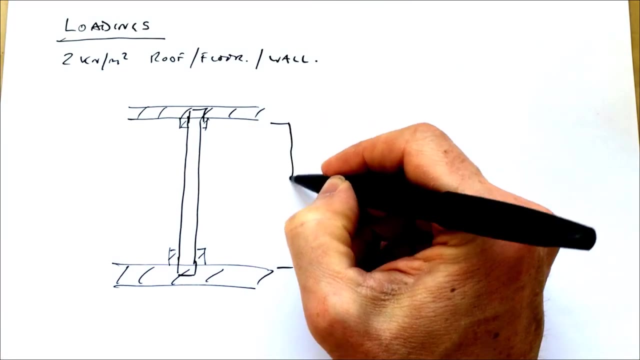 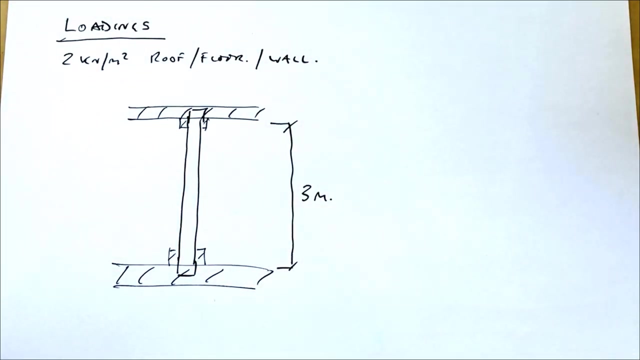 some masonry buttressing this wall at this location or at that location, And of course, we'll need to do padstone checks as well. So the distance between the supports here is going to be 3 meters in our example, And the floor. 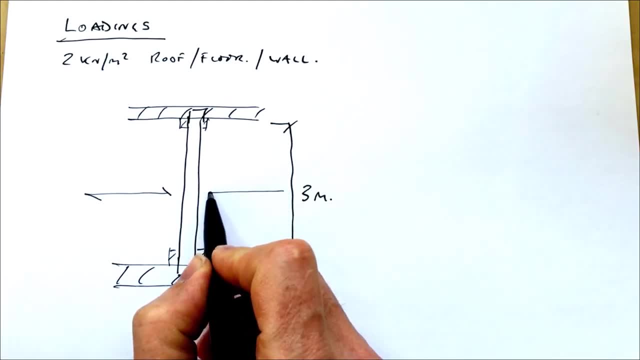 the first floor is spanning left to right onto the beam from one side and from the other side. Now, what we do is we take the midpoint of the floor at each side and that dimension, from midpoint to midpoint, is the area of load which is sitting on that beam. 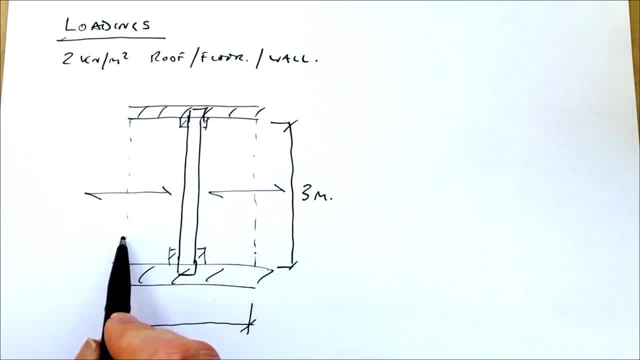 So that's the midpoint of this floor span and that's the midpoint of that floor span, And we're assuming that the floor is resting on another wall here and another wall there, So let's say this is 3 meters as well. Now, when working out the loadings on a beam, 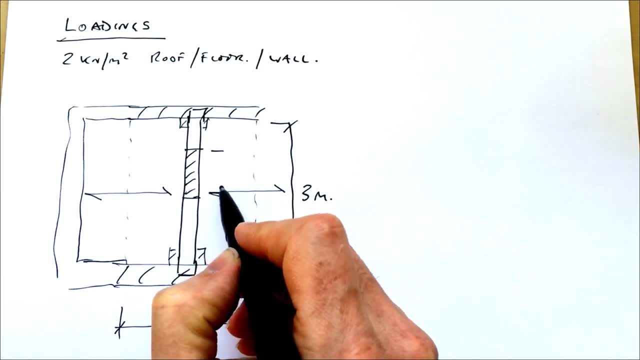 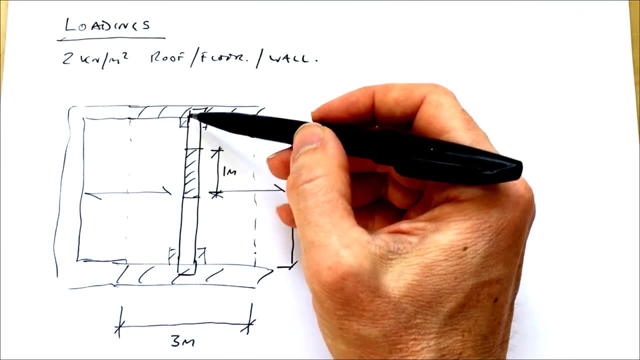 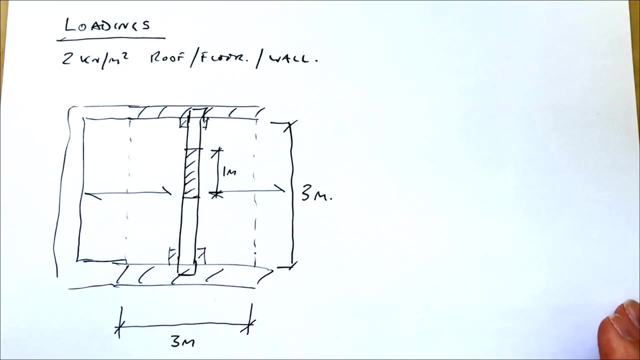 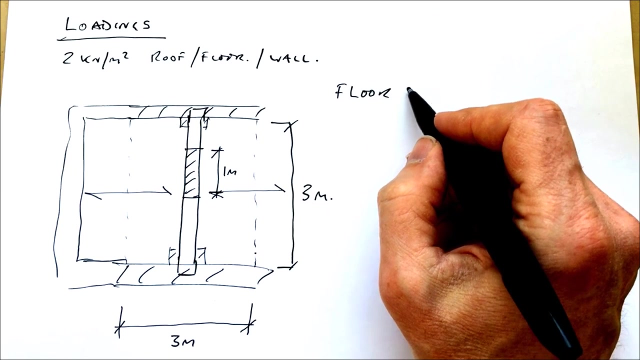 we're only interested in a meter section, because the loads that we're going to come out with are described as a load per meter, And I'll just explain how that works now. So for the floor, you've got 2 kN per meter squared of load. 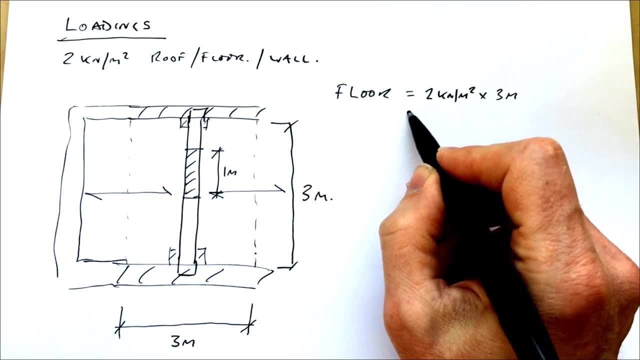 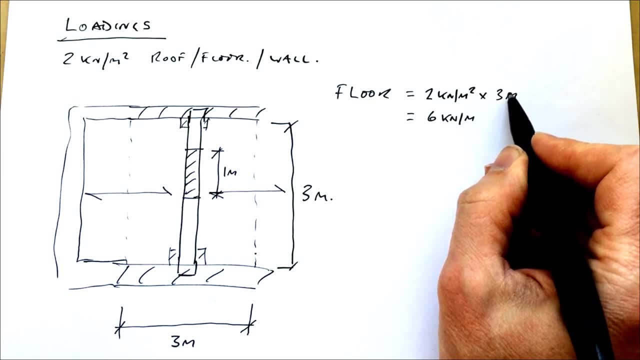 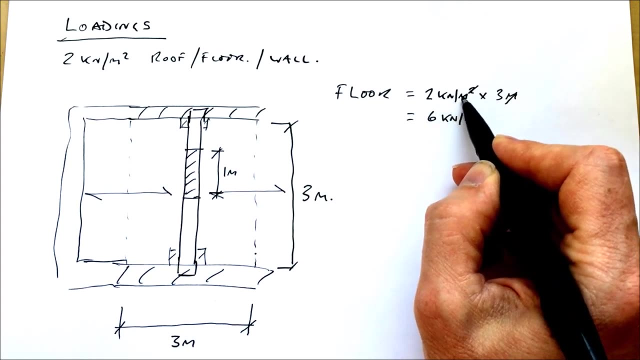 multiplied by 3 meters, which is going to give you 6 kN per meter, because that m and that m- one of those m's- cancel each other out. So you've got kN per meter left as your units, Just to repeat that. 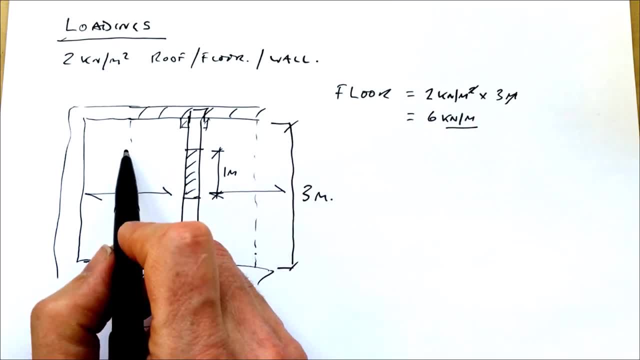 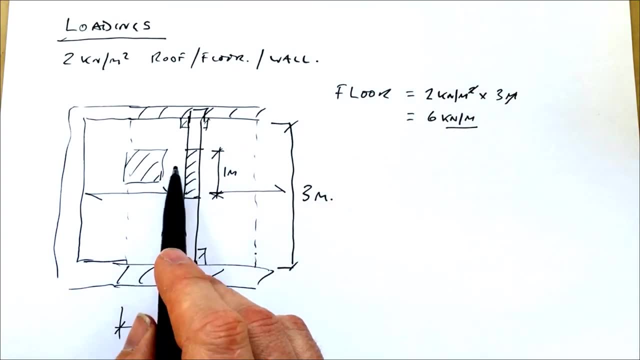 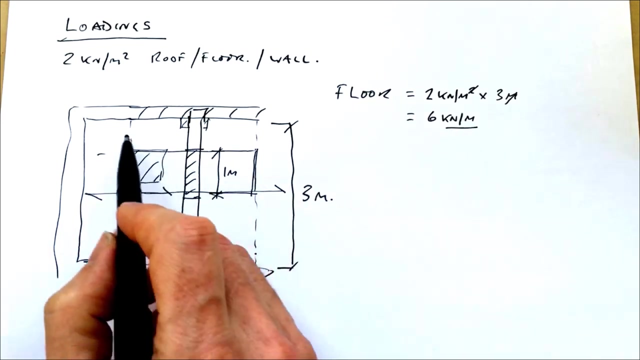 2 kN per meter squared. so that's for every square meter here there is 2 kN And we're having 3, lots of those acting on that part of the beam, which is this area here. Yeah, 1 meter by 3 meters. 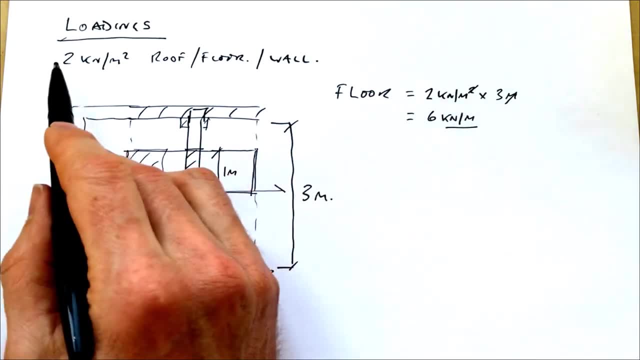 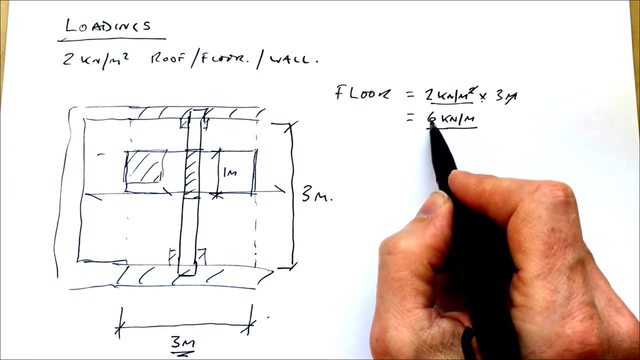 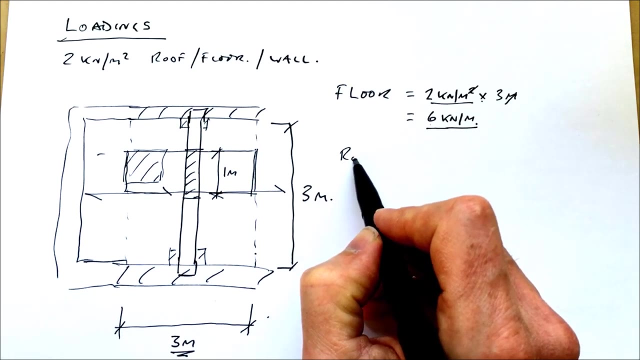 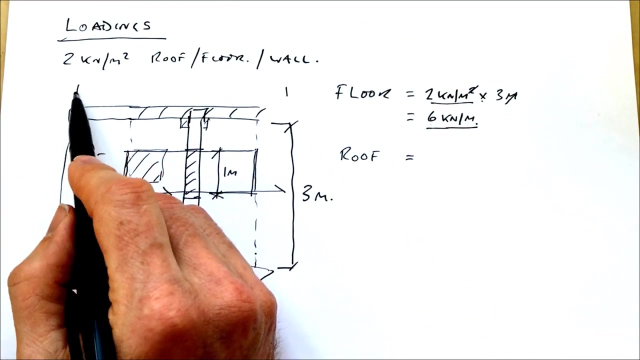 So we're taking our floor load, 2 kN per meter squared, and multiplying it by 3 meters to get to the answer of 6 kN per meter For the roof. we might have a similar thing happening because if the roof is spanning from here to here, 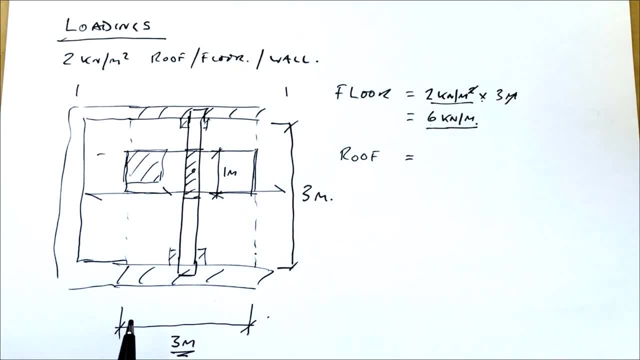 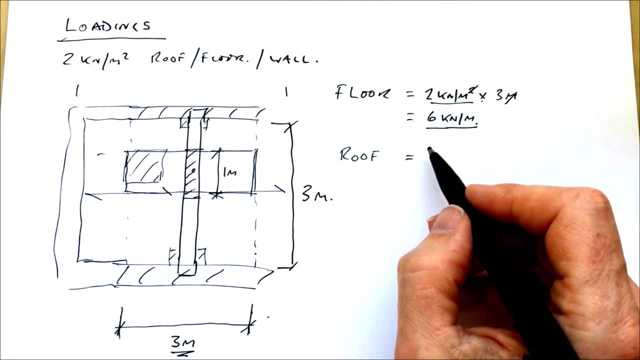 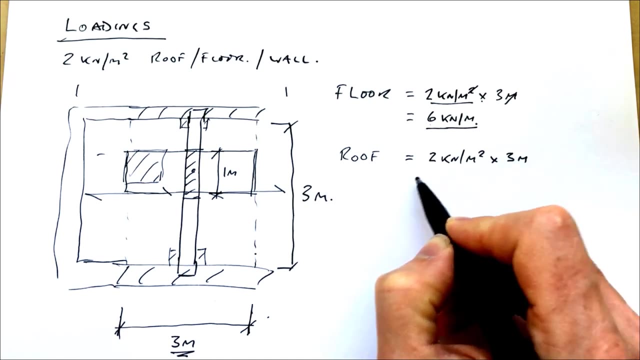 and it's propped over that beam, then again we're getting a 3 meter effective area of roof acting on that beam. So again the roof, we're going to say 2 kN per meter squared multiplied by 3 meters equals 6 kN per meter. 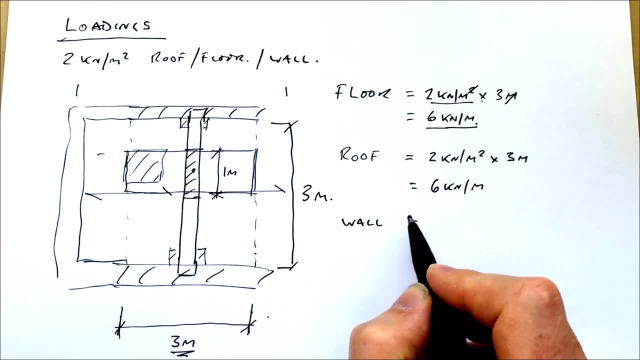 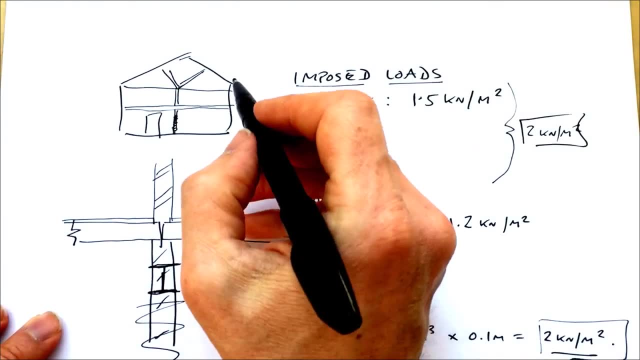 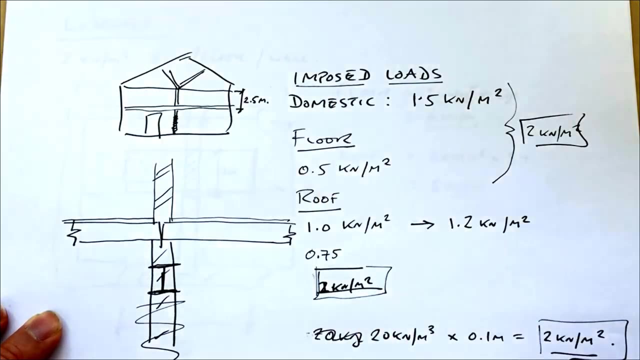 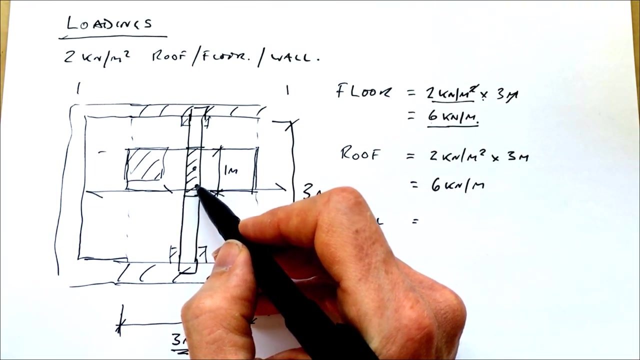 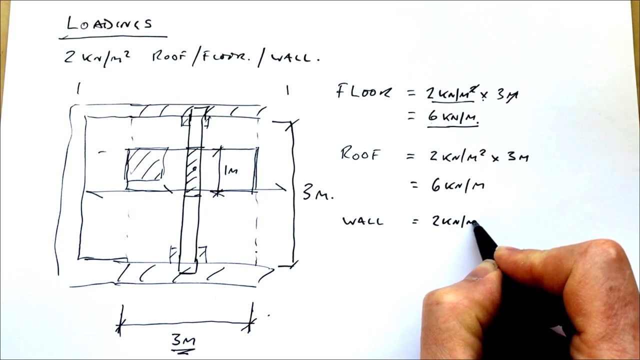 And the wall. going back to our sketch, here the wall height is going to be about 2.5 meters. So again for this meter length, here the load of the wall is going to be 2 kN per meter squared multiplied by 2.5 meters. 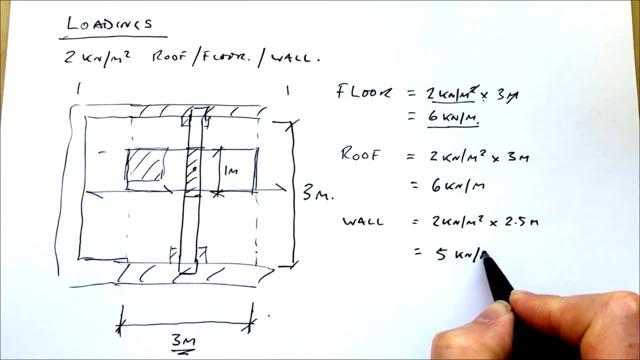 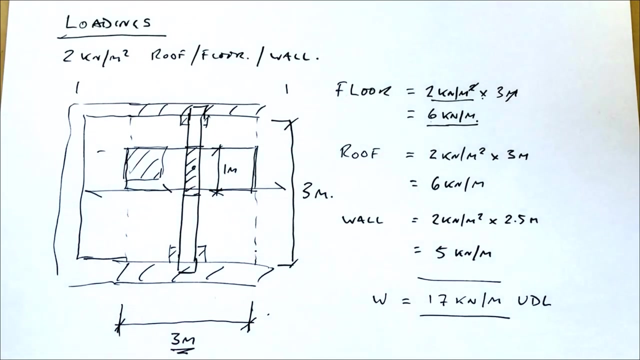 equals 5 kN per meter. So the total load acting on the beam is 6 plus 6 plus 5, which is 17 kN per meter. And that's the UDL and we'll call it W. So this is the load that we need to take. 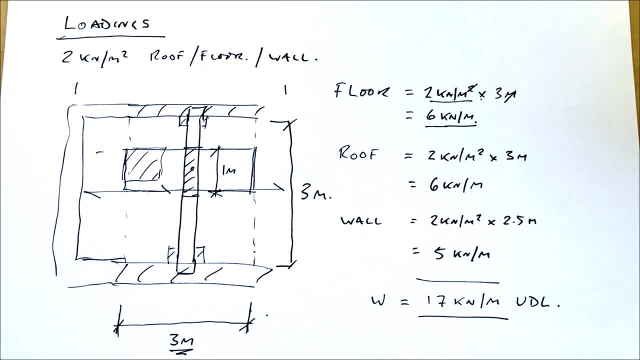 through into our beam design and we're going to sorry- into the beam analysis, which is the next video, and then we're going to do the beam design in the video afterwards, And the only thing to leave you with here is that we need a factor of safety.